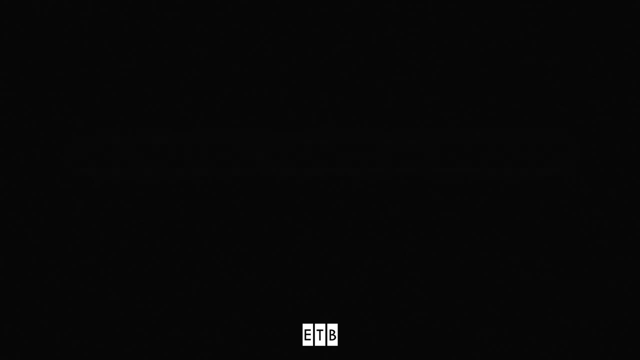 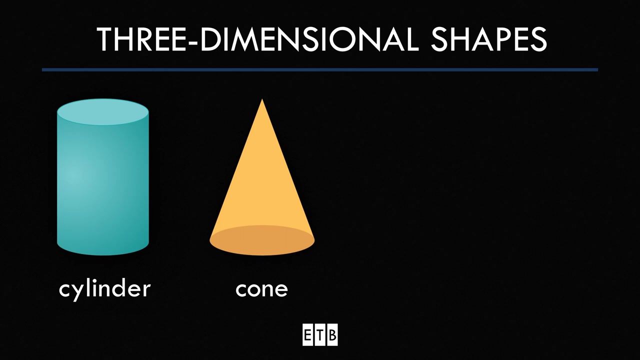 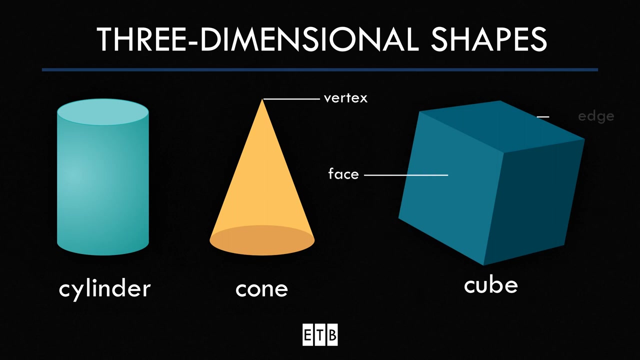 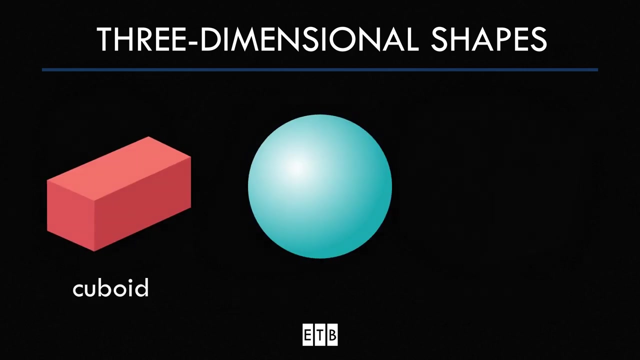 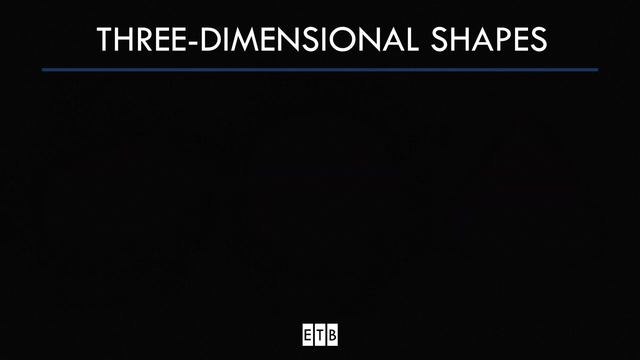 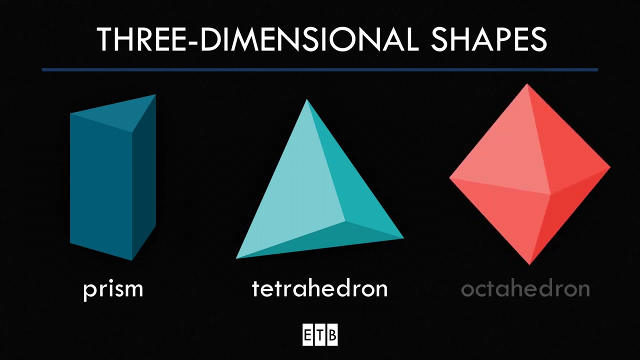 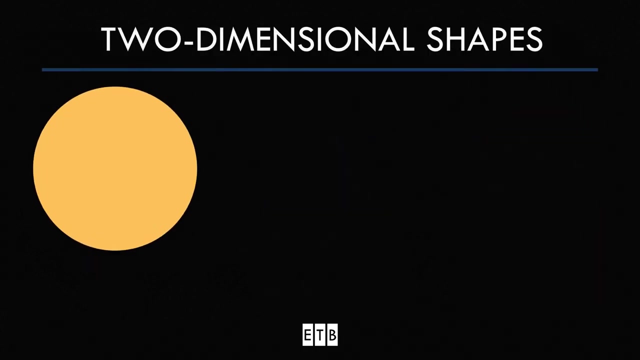 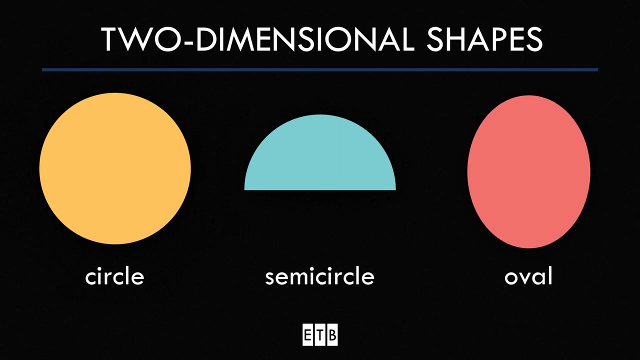 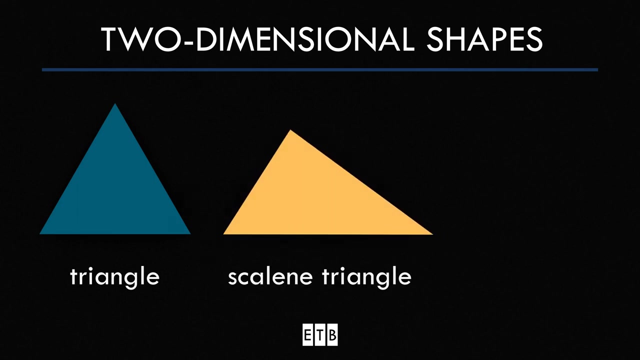 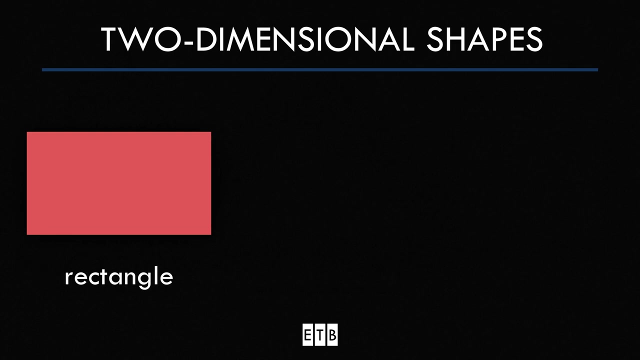 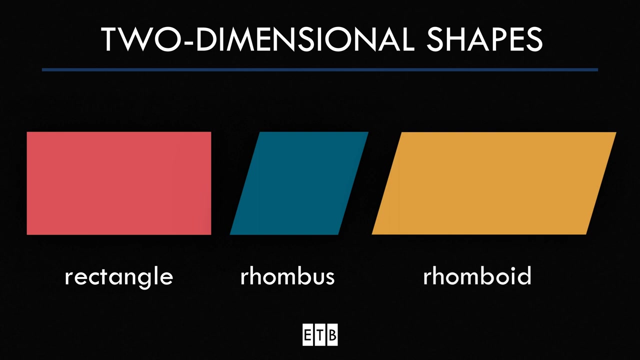 Geometric shapes in English. Three-dimensional shapes: Cylinder, Cone, Vertex, Cube, Face, Edge, Cuboid, Sphere, Pyramid, Prism, Tetrahedron, Octahedron. Two-dimensional shapes: Circle, Semicircle, Oval Triangle, Scapegoat, Teline Triangle, Square, Rectangle, Rhombus, Rhomboid. 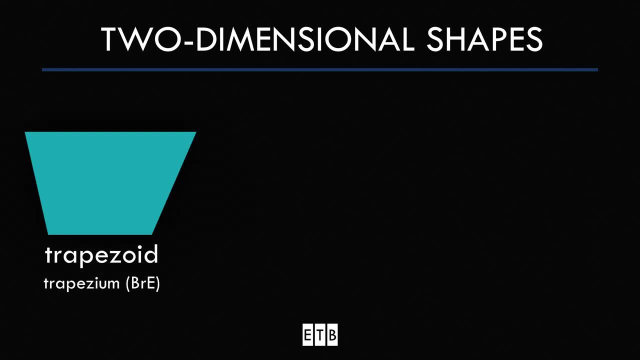 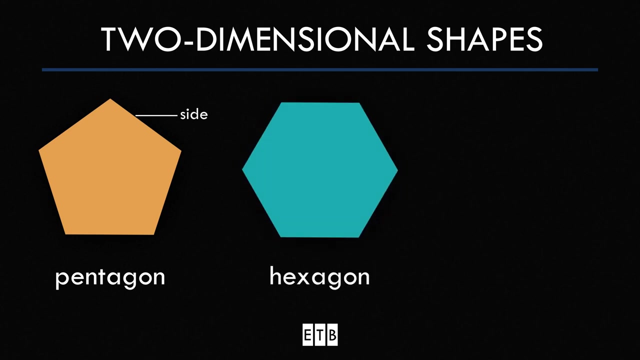 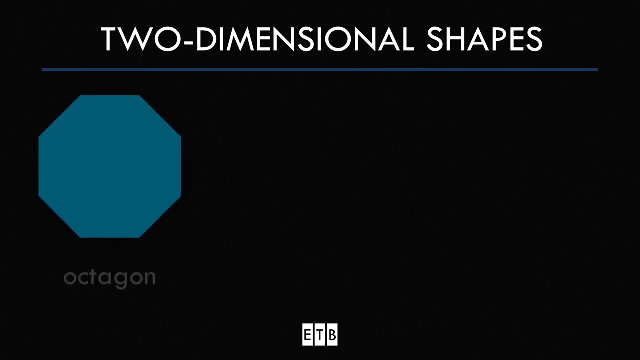 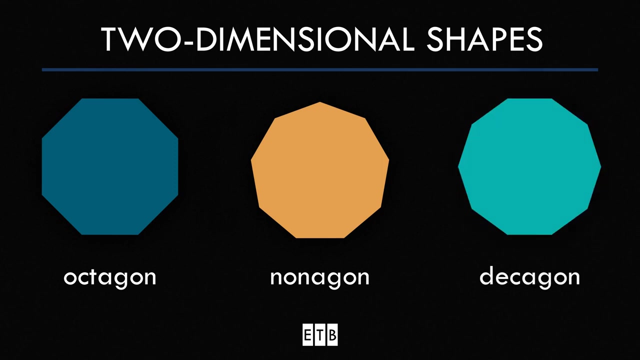 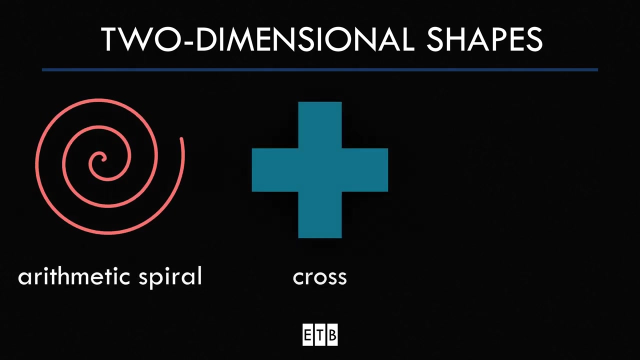 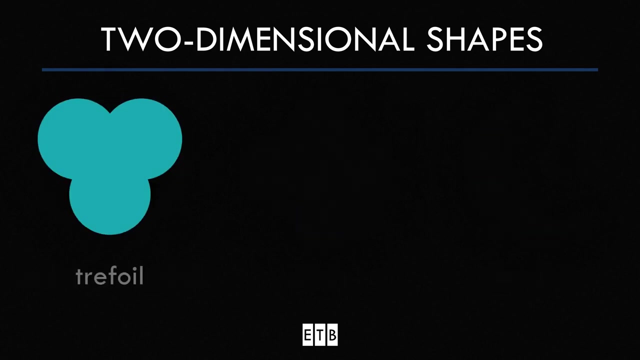 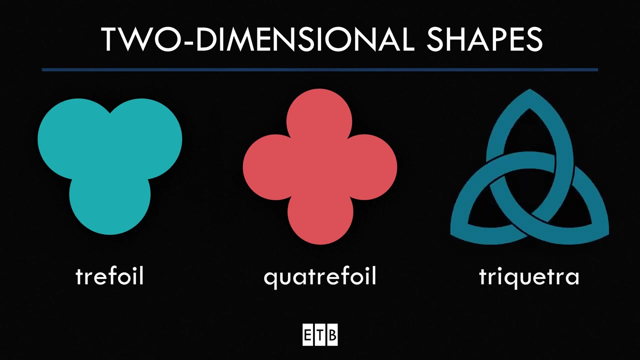 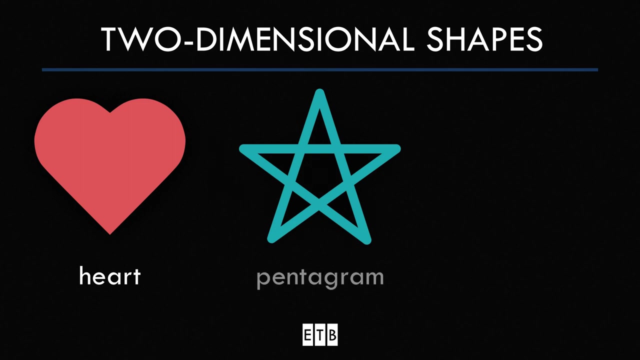 Trapezoid, Trapezeum, Trapezeum- kite, pentagon side, hexagon, heptagon, octagon, nonagon, decagon, arithmetic spiral cross: crescent trefoil quatrefoil triquetra heart- pentagram, pentagon- hexagram.